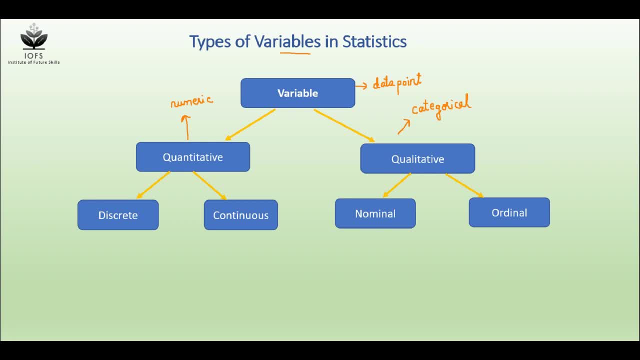 Let's see one by one what does each mean. Let's start with quantitative. Quantitative data are those data that are measurable or the ones you can measure or count. It means that you can do basic arithmetic operations like addition, subtraction, multiplication or division. 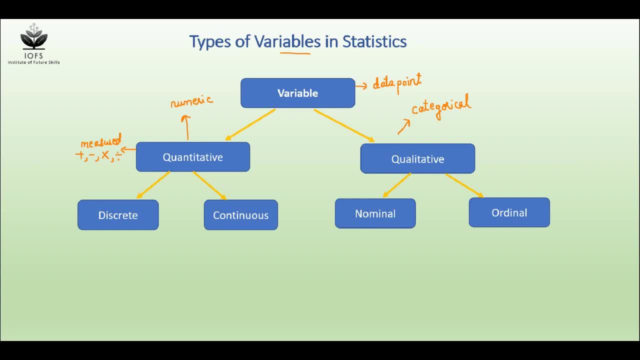 And the output makes perfect sense. Quantitative data is a data that is used to calculate the number of variables in a given data set. Quantitative data are further divided into two types. One is discrete and other is continuous. Discrete data are ones those take only particular values within a range. 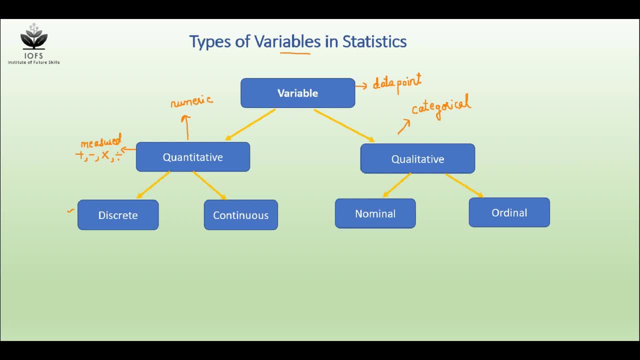 Let me give you an example so that it's clear. For example, it might be number of students in class. You can have 30 students, 40 students or 100 students. You can't have number of students as 30.5.. 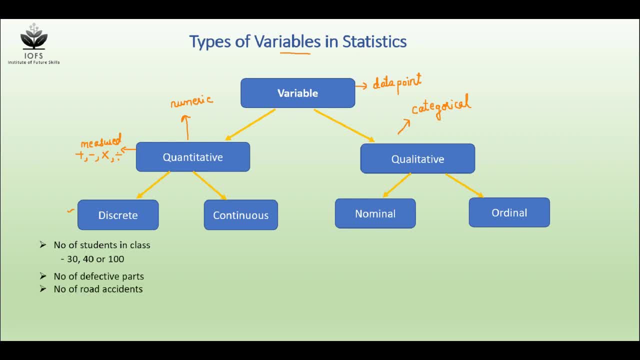 Other examples Of discrete variables would be number of defective parts that are manufactured in some company or a plant, or number of road accidents happening in a day. So discrete variables, or data point, are the ones that take only particular value within a range, Whereas when we talk about continuous class, they can take any value within a range. 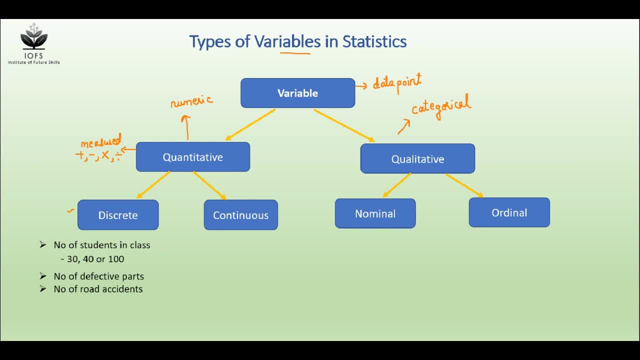 By saying any, I mean they can take uncountable number of values within a range. Example Would be weight. You can have weight as 68.45 kg. You can have it as 68.456 or 70.5.. 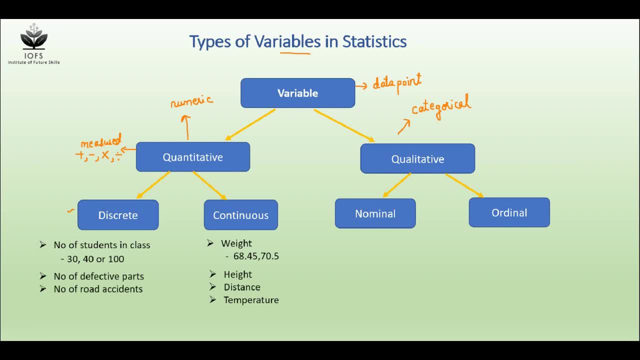 Other examples would be height, distance, temperature, because these variables have decimal values. So I think you're clear with quantitative data. Let's check what does qualitative data means. Qualitative data are descriptors or characteristics that cannot be easily measured. Qualitative data are descriptors or characteristics that cannot be easily measured. 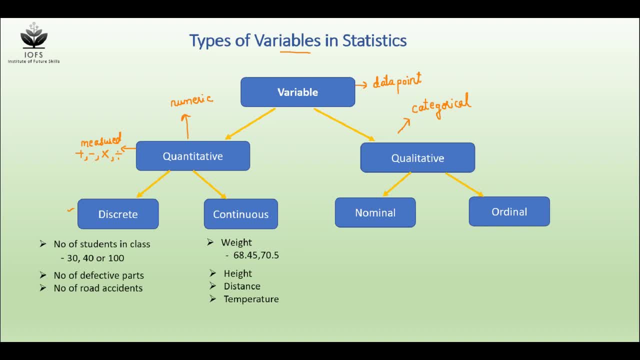 But they can be observed, like taste, smell, etc. Qualitative data are divided into two parts. One is nominal and other is ordinal. Nominal data have names or labels associated with it And they do not have any order. So you should remember there is no intrinsic order in nominal data. 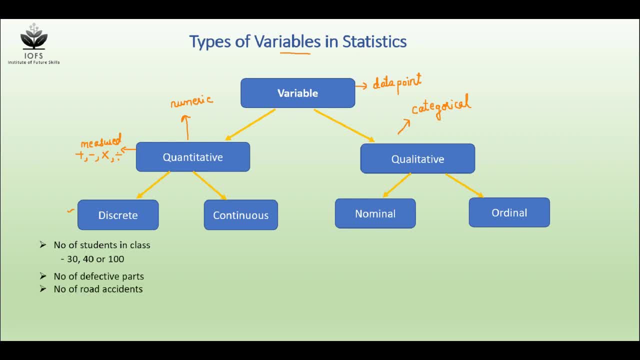 Other examples Of discrete variables would be number of defective parts that are manufactured in some company or a plant, or number of road accidents happening in a day. So discrete variables, or data point, are the ones that take only particular value within a range, Whereas when we talk about continuous class, they can take any value within a range. 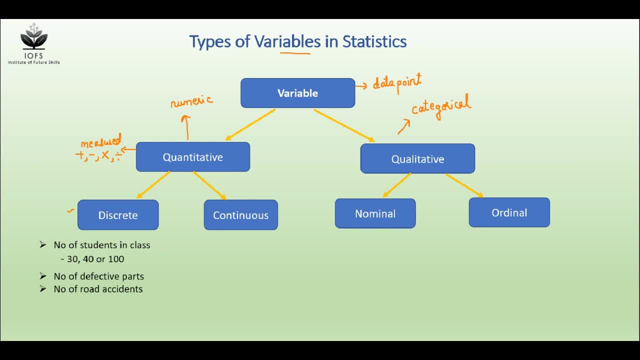 By saying any, I mean they can take uncountable number of values within a range. Example Would be weight. You can have weight as 68.45 kg. You can have it as 68.456 or 70.5.. 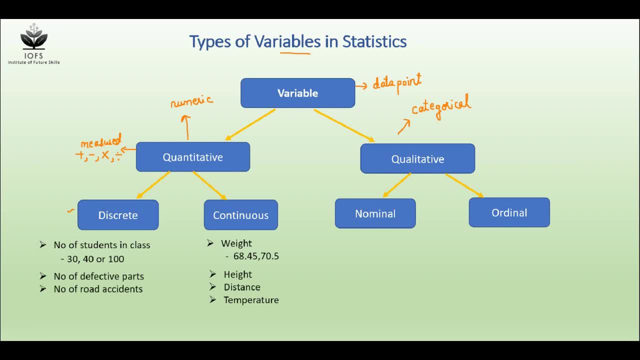 Other examples would be height, distance, temperature, because these variables have decimal values. So I think you're clear with quantitative data. Let's check what does qualitative data means. Qualitative data are descriptors or characteristics that cannot be easily measured. Qualitative data are descriptors or characteristics that cannot be easily measured. 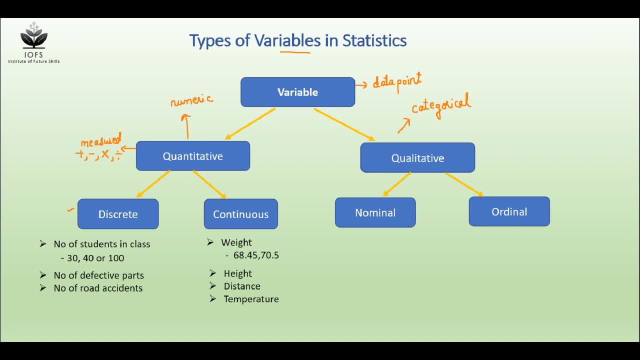 But they can be observed, like taste, smell, etc. Qualitative data are divided into two parts. One is nominal and other is ordinal. Nominal data have names or labels associated with it And they do not have any order. So you should remember there is no intrinsic order in nominal data. 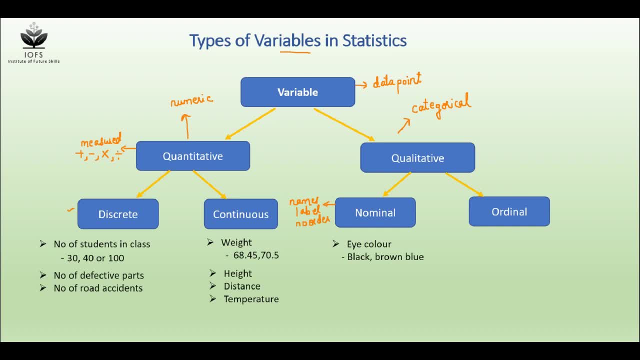 For example, Eye color. You can have black eye, brown eye or a blue eye. Other examples would be blood group state and zip code. State and zip code are labels that are usually given for geographical locations, Whereas when we see ordinal data, the variables are ordered. 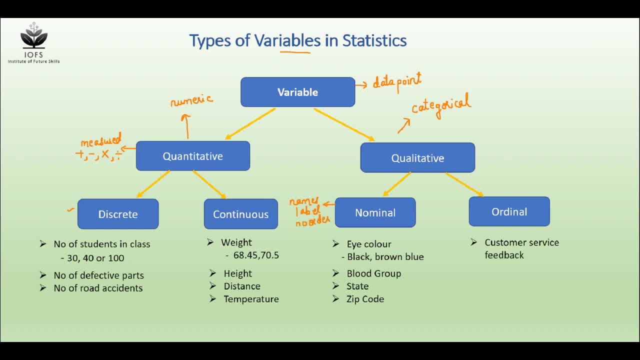 For example, you might have a feedback from your favorite restaurant where they're asking you to rate the customer feedback. So you'll rate that. So you have to rate them on a scale like 1 being poor, 2,, 3,, 4,, 5, and 5 being excellent. 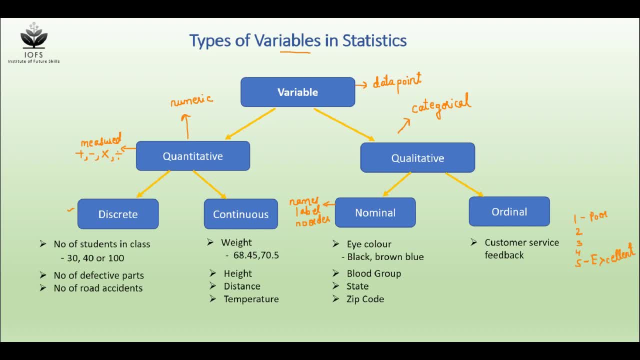 So you have to rate them on a scale from 1 to 5.. Other examples would be ranks for students. So ordinal data have ordered. I hope you're clear with types of variable and its kind. Let's go ahead and see one data set. 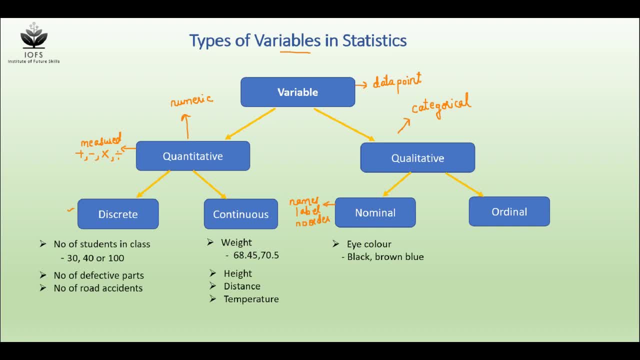 For example, eye color. You can have Black eye, brown eye or a blue eye. Other examples would be blood group state and zip code. State and zip code are labels that are usually given for geographical locations, Whereas when we see ordinal data, the variables are ordered. 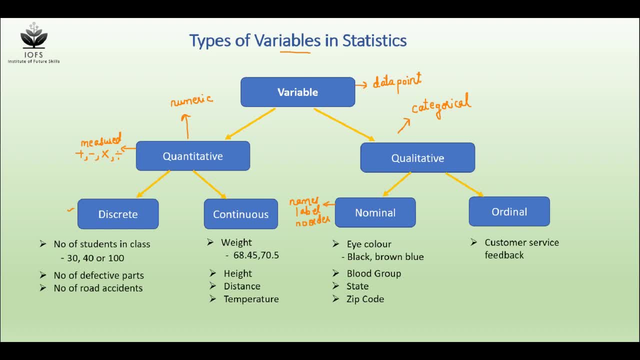 For example, you might have a feedback from your favorite restaurant where they're asking you to rate the customer feedback. So you'll rate them on a scale Like one being poor, two, three, four, five and five being excellent. So you have to rate them on a scale from one to five. 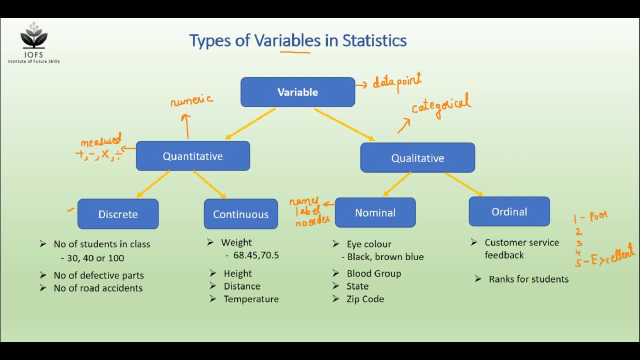 Other examples would be ranks for students. So ordinal data have ordered. I hope you're clear with types of variable and its kind. Let's go ahead and see one data set Where we will see each kind of variable and what are its type. 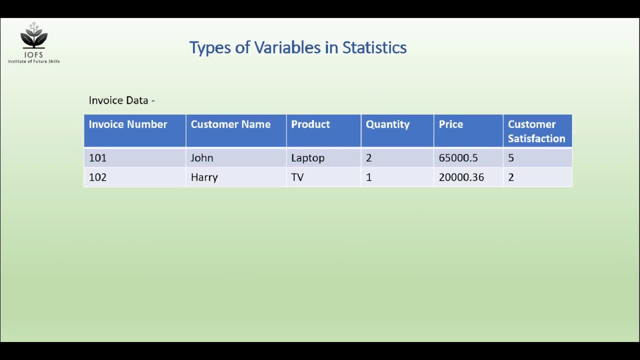 So this is invoice data. Let's see what columns it has. You have invoice number, customer name, product quantity, price and customer satisfaction. Let's see what kind of variables we have. So invoice number, customer name and product. 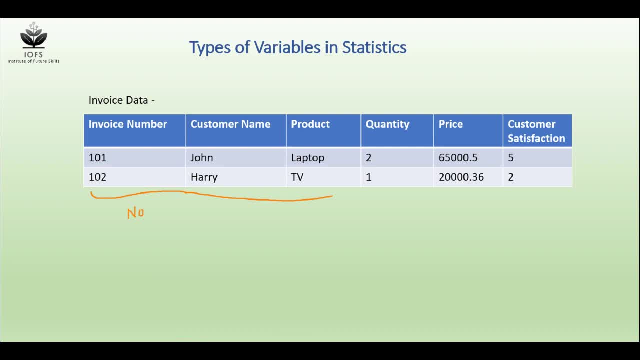 These are nominal data, Which is kind of qualitative data, Quantity being of discrete data, Because it does not have any decimal point. Price is continuous And customer satisfaction is ordinal data, which is a type of qualitative data. So I hope you're clear with types of variables in stats. So let's go ahead and see one data set. Let's see what kind of variable we have. So ordinal data has ordered. Let's see what kind of variable we have. Let's see what kind of variable we have. Let's see what kind of variable we have. 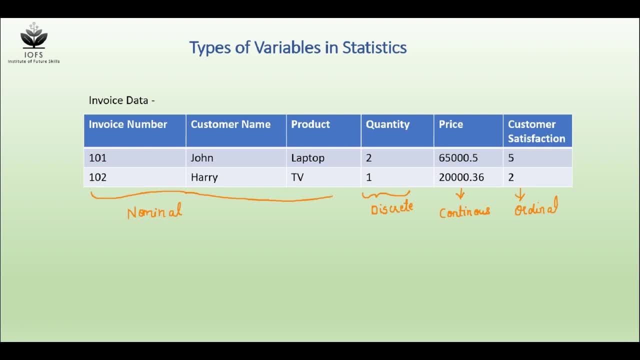 like this video. please like and subscribe to my channel. thank you for watching this video. happy learning.